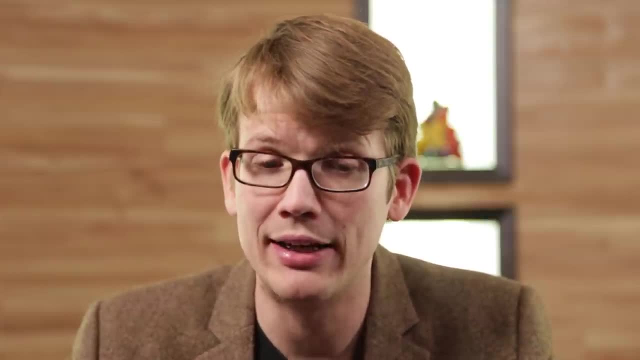 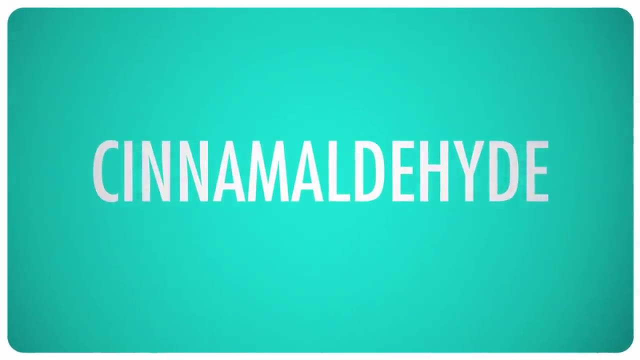 And, yeah, I hated my mom for like a full year after that, but she was right, That girl was trouble. So, yes, you are allowed to hate IUPAC for changing the name of cinnamaldehyde- the aldehyde that makes cinnamon smell like cinnamon- to trans-3-phenylprop-2-anol. 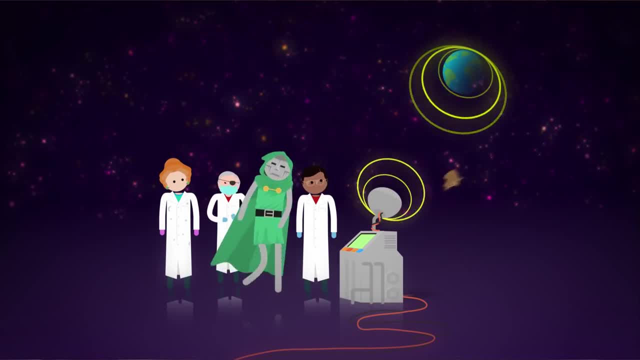 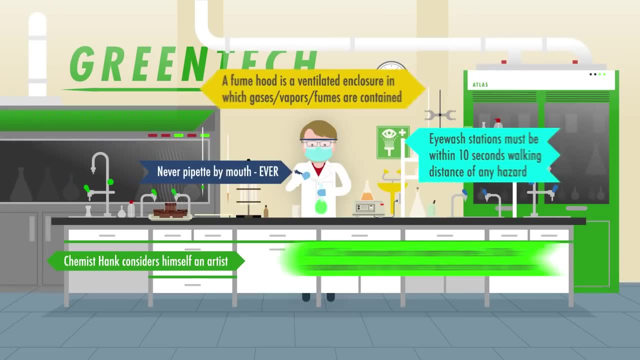 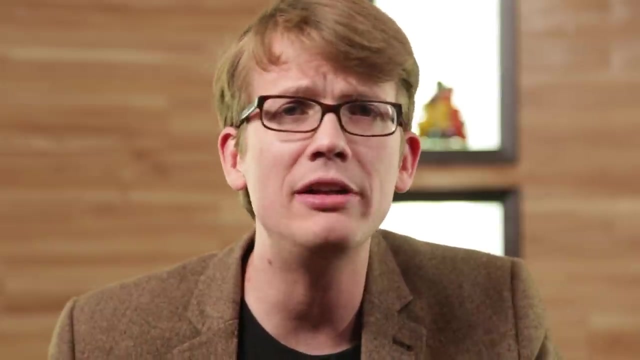 Yes, they're sucking all of the fun out of the world, but trust me when I say they're doing it for your own good. CINNAMALDEHYDE: Cinnamaldehyde is a lovely name for a lovely aldehyde, just like cadaverine is a creative name for a rancid-smelling amine. Citronellol, angelic acid, vanillin- they're beautiful names, but there are tens of thousands of regularly used organic compounds, and we can't come up with pretty names for all of them. More important than that, though, there's no way to translate those names into chemical formulas. And IUPAC hates that. They're like cinnamaldehyde. Sure, it gives cinnamon its lovely smell, but we think that trans-3-phenylprop-2-anol is way better of a name. And it actually is, because if I say trans-3-phenylprop-2-anol to somebody properly educated, they can just write down the chemical structure without even thinking about it. 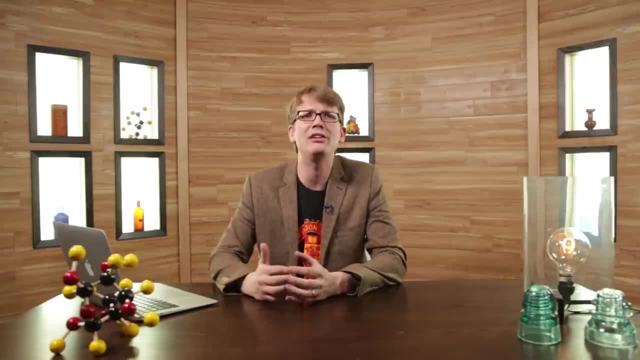 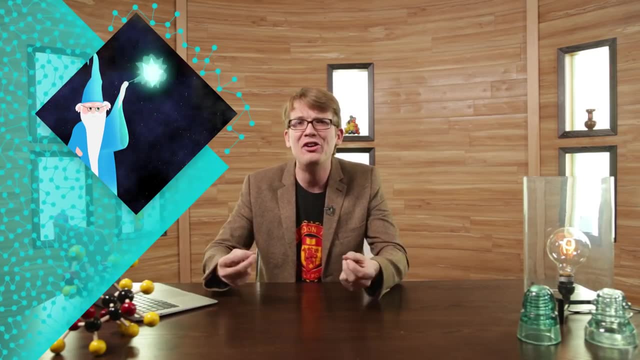 And that's like almost a kind of magic, where words go from relating to reality as we experience it- this chemical comes from cinnamon, so name it after cinnamon- to relating to the actual physical reality of the universe, And that's a magic worth knowing. 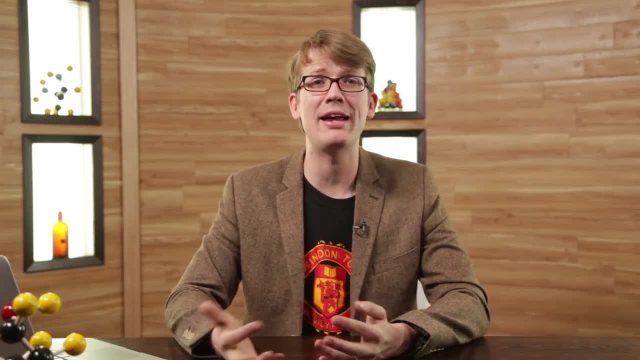 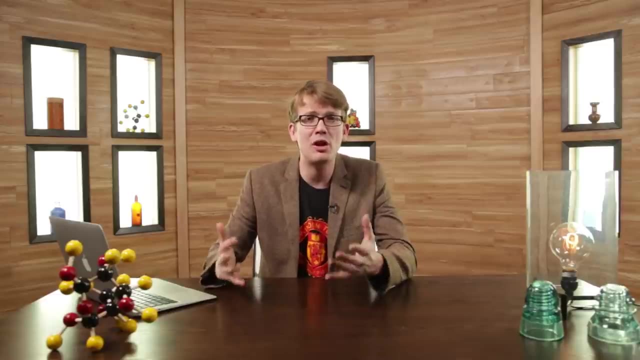 IUPAC created a language that could be understood, A language that could be understood by everyone, with minimal, even zero, misinterpretation, And that's no easy feat. That's why, as we've discussed organic chemistry, when we start counting carbons, we make sure that the first thing named on the molecule is the lowest possible carbon. 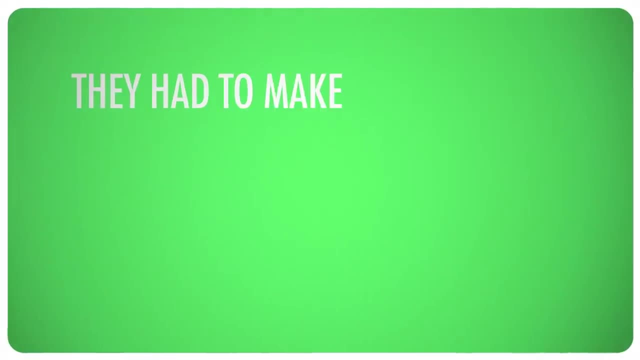 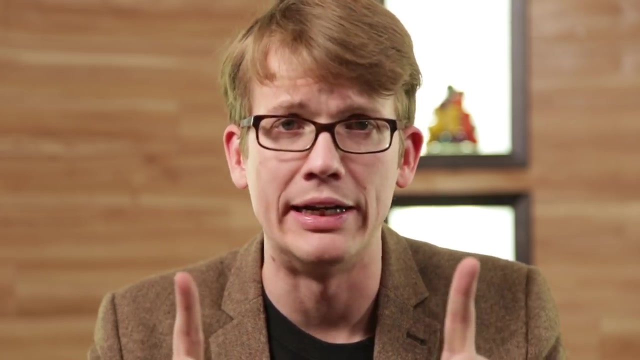 Not because there's something special about lower numbers, but because they had to make a rule, otherwise one chemical could be named two different ways. Let's go through the process of naming a chemical. It's a multi-step process. Step one: How long is the carbon chain? 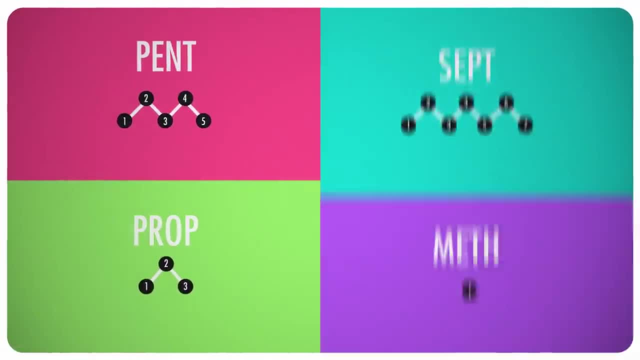 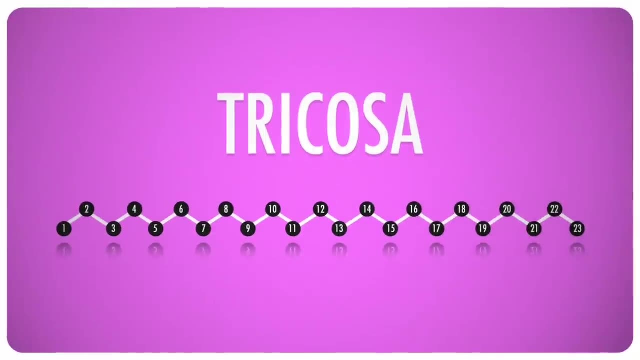 Five carbons will have pent, seven sept, three prop one meth. Don't feel weird if you have to look these up. I, for example, had no idea that a 23 carbon atom chain had the prefix tricosa until I looked it up just now. 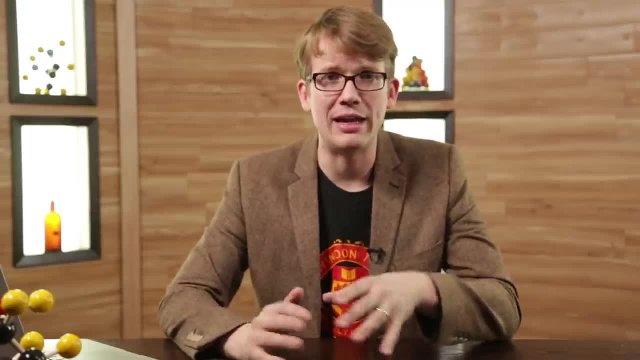 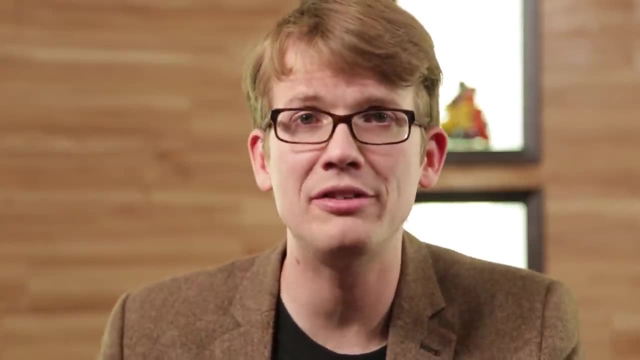 The only tricky thing here is to make sure you find the longest carbon chain. Sometimes a hexane can look like a pentane with an ethane sticking off of it. So now that you know your longest carbon chain, you've got your prefix. time to figure out the suffix. If there's nothing but hydrogen and carbon, your suffix just depends on whether you have any double bonds or triple bonds. You know these: Propane, propene, propine. Then there are a ton of other groups that can change the suffix. 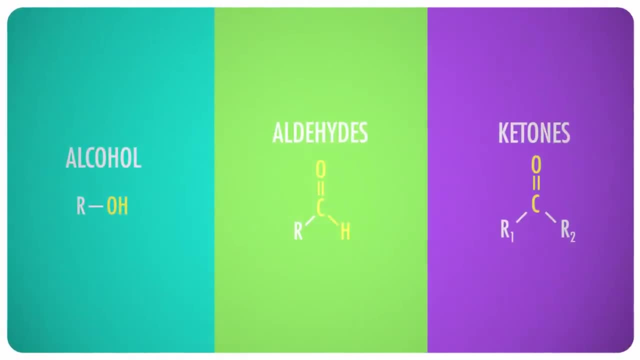 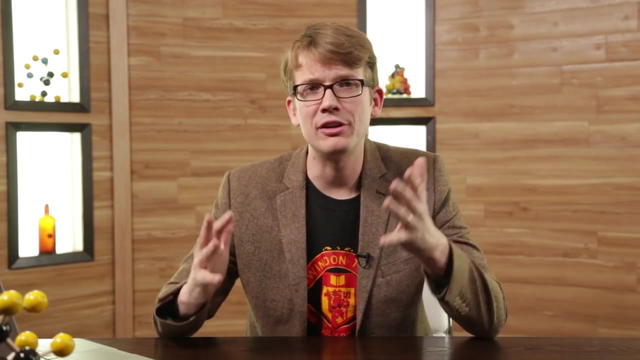 Like last week. we talked about alcohols and aldehydes and ketones, but we didn't talk about how they affect nomenclature. and boy do they When working with functional groups. each one adds a particular suffix to the end of the name of a compound. 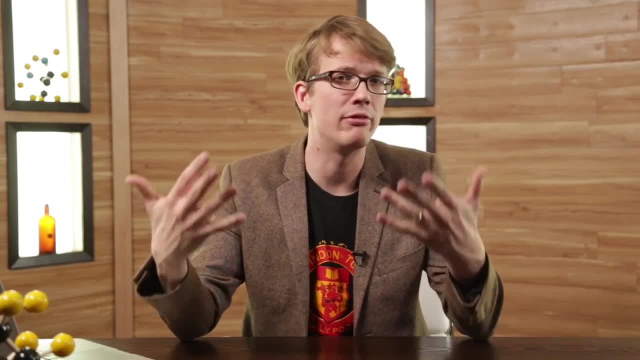 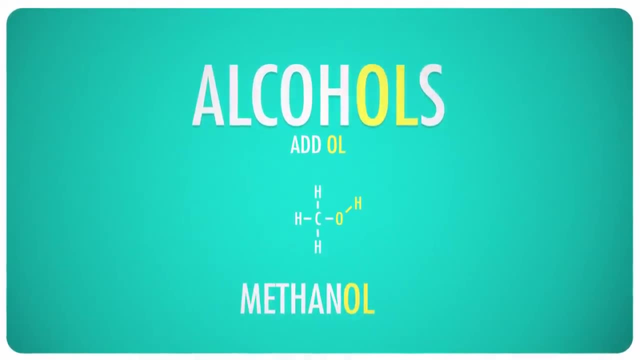 Usually these are pretty easy to remember because they come straight off of the name of the functional group. Alcohols: add an OL. so for methane you drop the E and you get methanol. Ethane, you get ethanol Aldehydes. instead of OL, you add AL. 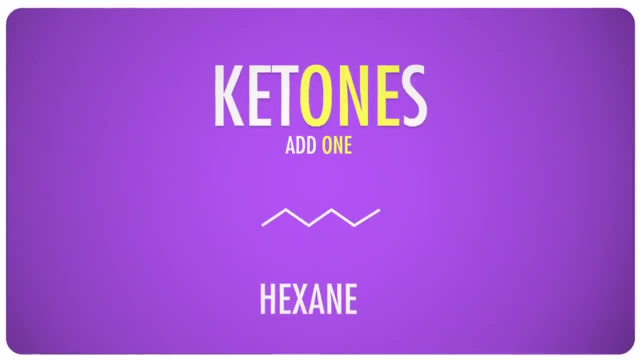 So from ethane you get ethanol Ketones add ON, so a ketone of a hexane would be a hexanone And amines- you just add amine to the end, So methanamine or propanamine, super easy. 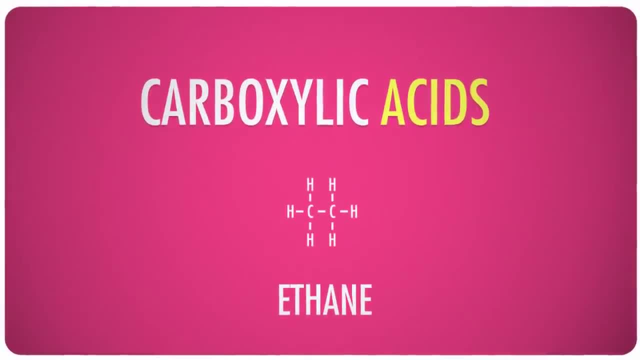 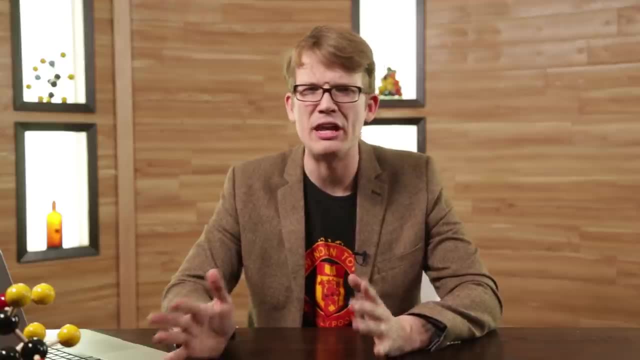 For carboxylic acids you have to identify that it's an acid. so you end in acid. That's obvious. But instead of adding ilic, you add oic. As far as I can tell, this is just because ethanoic acid is much more fun to say than ethanilic acid. 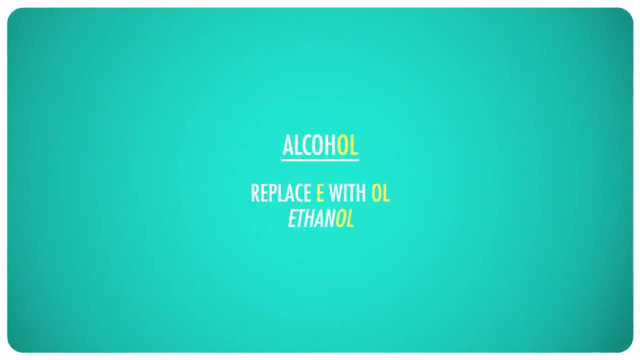 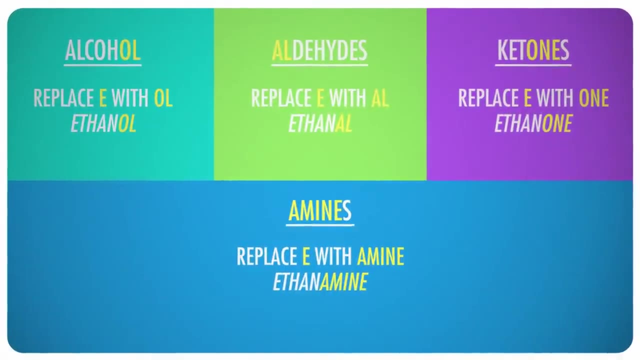 Going over that again. Alcohol on an ethane is ethanol Aldehydes- add AL giving ethanol Ketones. add O in E Pronounced ethanone Amines, add amine for ethanamine. And carboxylic acid on an ethane is ethanoic acid. 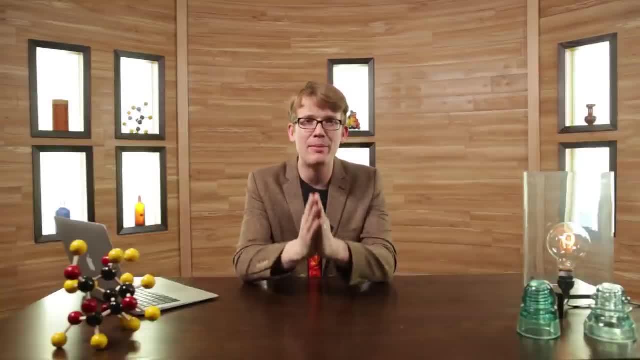 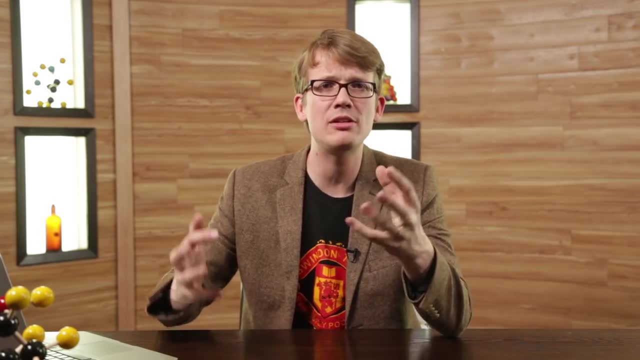 And of course there are literally dozens of other named functional groups that will change the suffix. It's terrible. That's why they're on Wikipedia. So if you've got a functional group, there's a name that defines the suffix of the molecule. 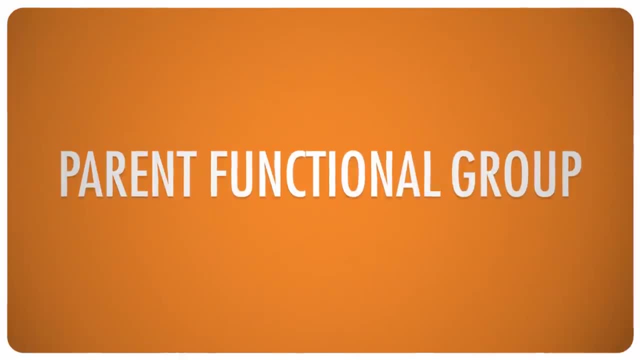 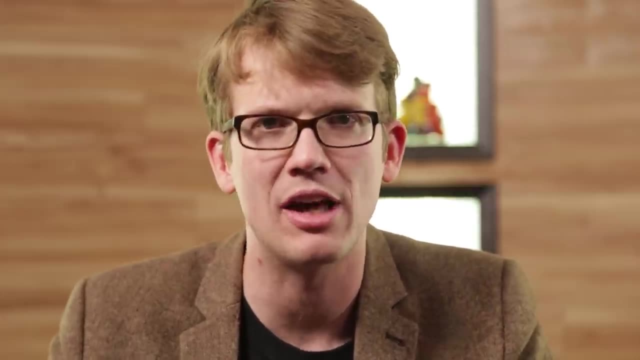 And that is called the parent functional group. Now, it is perfectly possible that a molecule will have two different functional groups. So how do we know which one is the parent, Which one defines the suffix? Well, different groups have different names. Precedence. 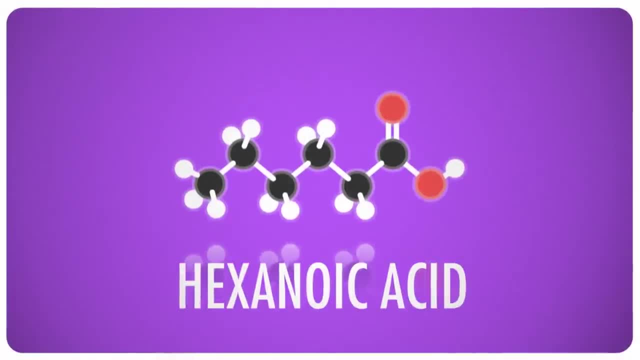 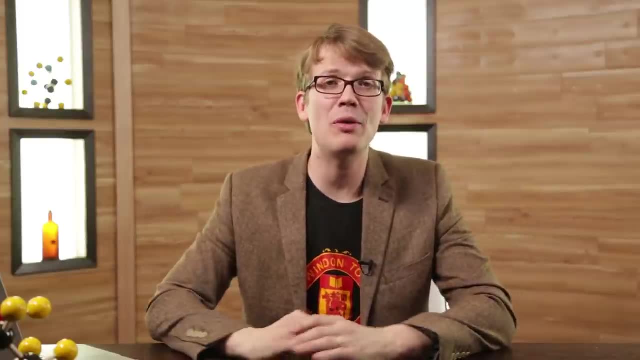 The most weighted of all is the carboxylic acid functional group. So no matter what else is on a six-carbon chain, if there's a carboxylic acid, then it's a hexanoic acid. That precedence is decided by a list. that was, you guessed it- created by IUPAC to minimize confusion by creating yet more rules. 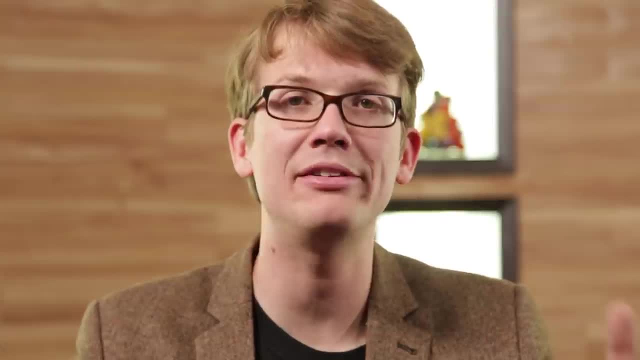 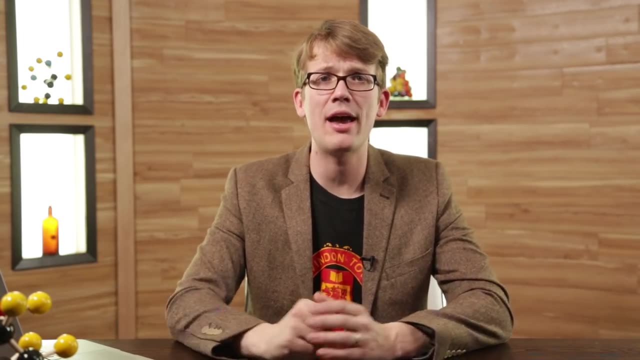 The list is linked in the description. Okay, so now we have created our base name for the molecule, It's time to start looking at what else is attached to it. Any side chains or functional groups sticking off the side have to be identified and named. 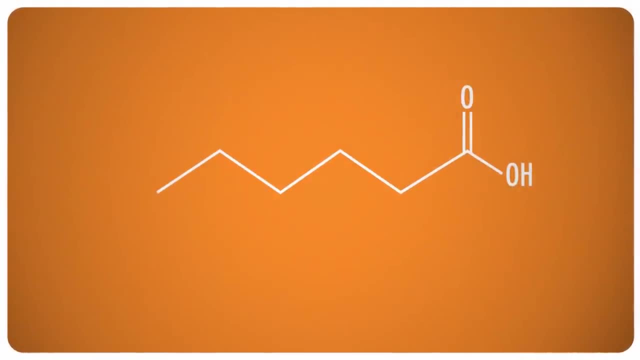 If it's a six-carbon chain with a carboxylic acid on it and an alcohol on one of the other carbons, our name has to do two things: Identify that the hydroxyl group is there and identify where it is. 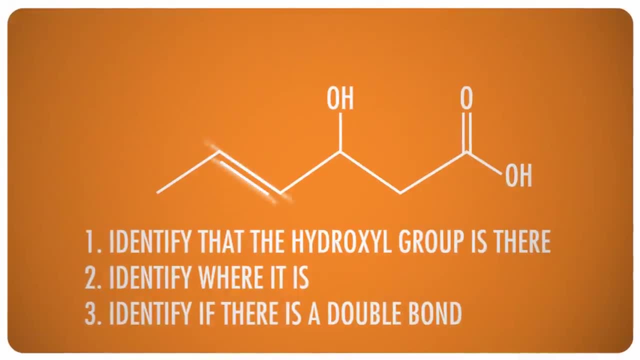 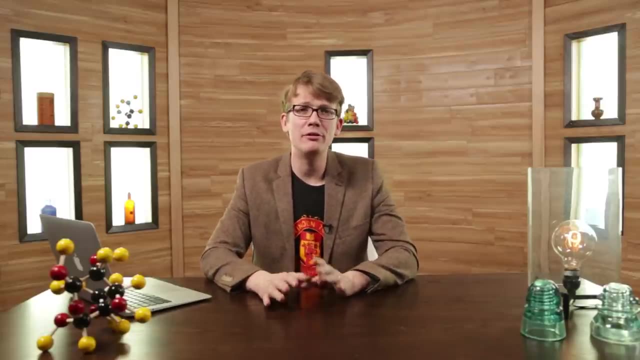 If it's got a double bond, we likewise have to identify that it is there and where it is. All with our words. Use your words. Also, use your numbers. Counting out carbons can be a little confusing, but try it both ways, in both directions, to make sure you get the lowest possible number on the group that defines your suffix. 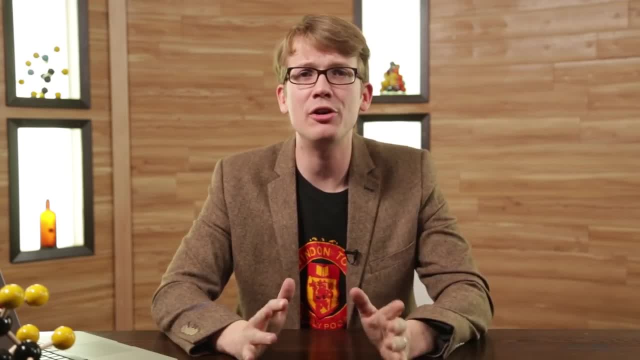 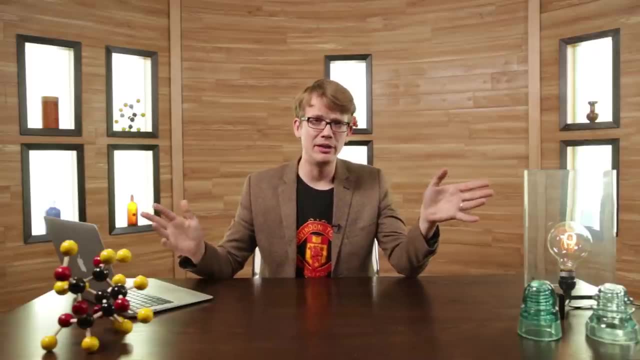 All right, enough of the talking, Let's try to do some actual examples here. I mentioned earlier angelic acid. It's not actually particularly angelic, It's just named after a flower that it was derived from, But it's actually all over the place in nature. so angelic acid tells us pretty much nothing about the molecule, except that it's acidic. 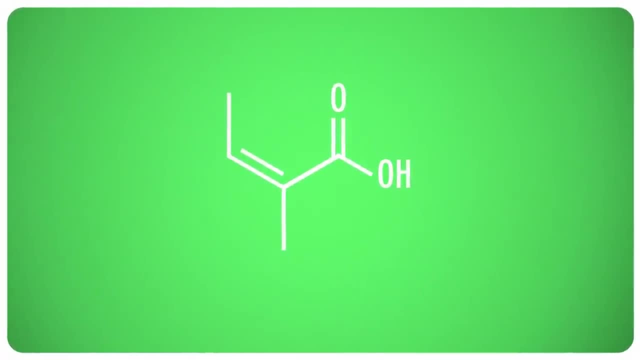 So, in order to figure out the structure, I have to look it up. That's no fun, but here it is. Let's figure out a better name for it. Count out the carbons One, two, three, if you count that chain. 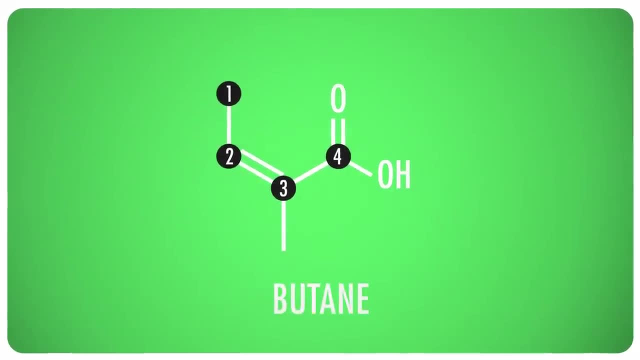 One, two, three, four if you count this one, So it's a butane derivative. Actually, it's a butene derivative because it has that double bond. It's also got the carboxylic acid though, so let's go ahead and call it butanoic acid. 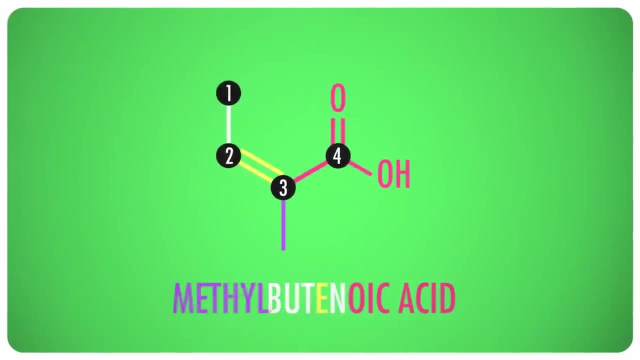 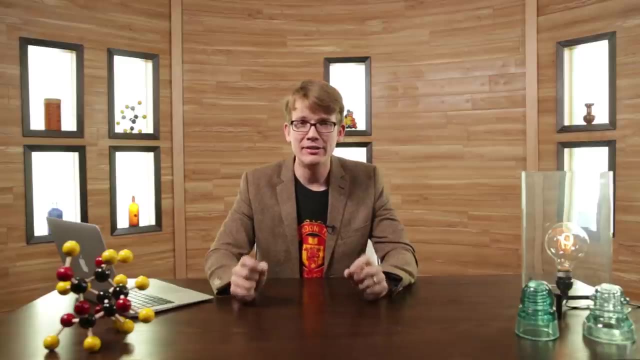 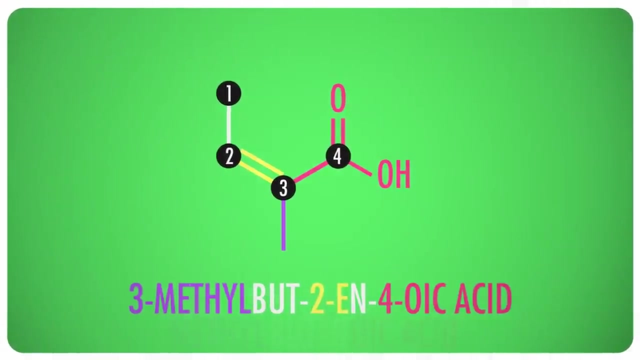 Except that there's a methyl group sticking off. so it's methylbutanoic acid, Of course with that name, without any numbers. no one has any idea where anything is on the chain. so time to number. From this direction- one, two, three, four, we get 3-methyl-but-2-in-4-oic acid, which is obviously wrong. 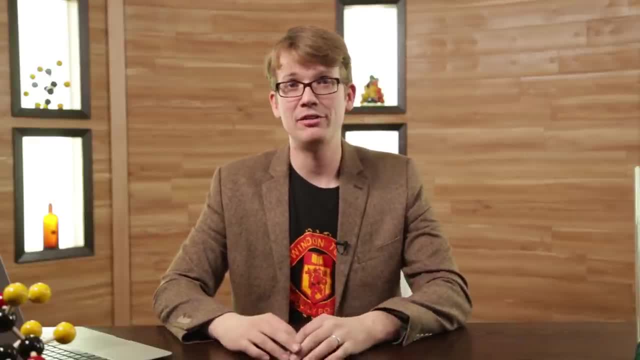 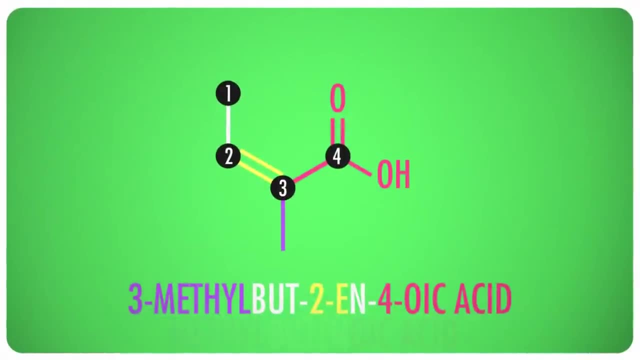 Mostly because that parent functional group, the one that defines the suffix, is supposed to be as low as possible, And in fact it is as high as possible, so that can't be wrong. Also, it just sounds terrible Numbering the other way: one, two, three, four. the carboxylic acid is on carbon one. 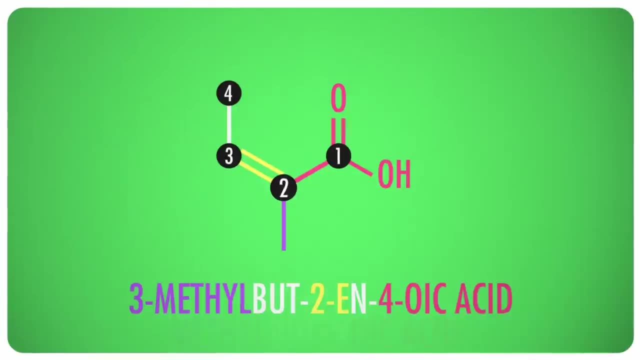 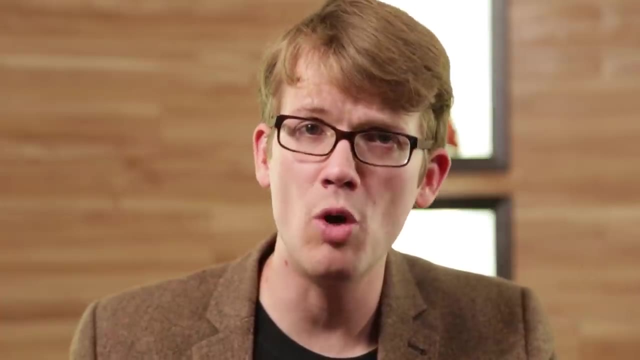 That's pretty ideal. The double bond and the methyl group are both on the second carbon much better, and thus it is named 2-methyl-but-2-in-4-oic acid. Two important notes here: If a parent functional group is on carbon one, we just leave the number off. 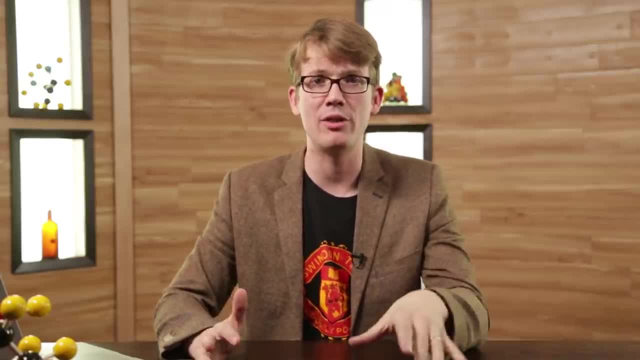 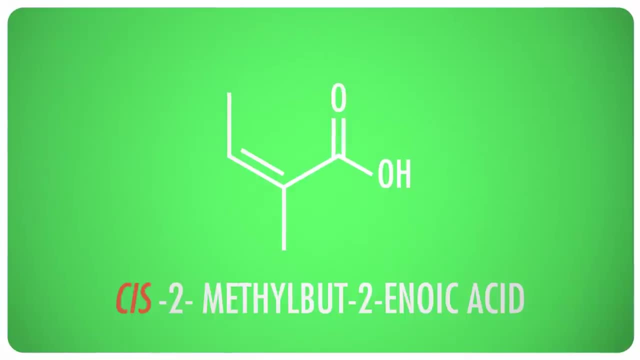 And two, there's a double bond in this molecule and we haven't identified whether it's cis or trans, And we can't do that, so we haven't actually completely named it. We should stick a cis in front of the name, because the carbon chain continues on the same side, not the opposite side. 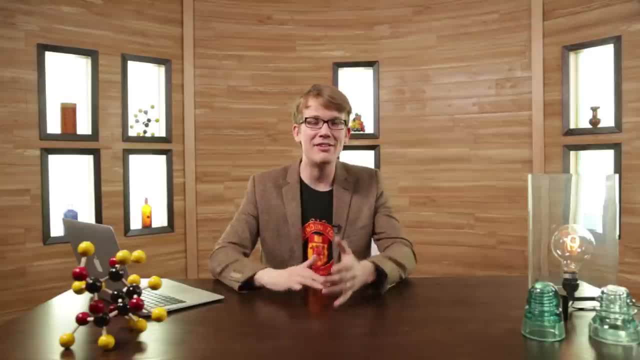 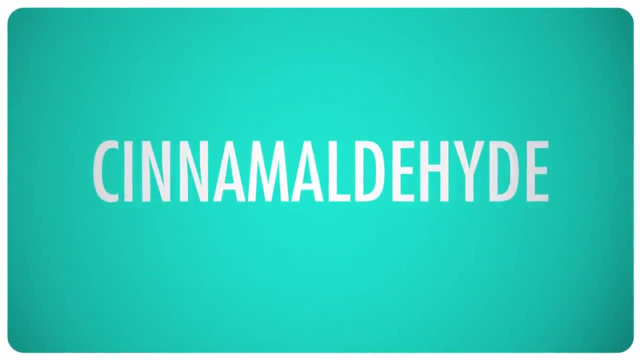 as it would be in the trans form. Of course, it works both ways. That's the beauty of it: You can build a name from a molecule and a molecule from a name. Earlier, I told you that cinnamaldehyde was trans-3-phenyl-prop-2-in-all. 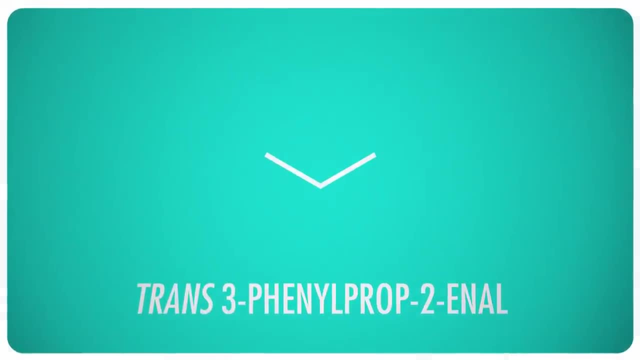 Can you build it? Well, start with a three-carbon chain because of that prop and count out the carbons One, two, three. We know because it's prop-2-in-all with that E there's a double bond from the second to third carbon and we know it's trans.